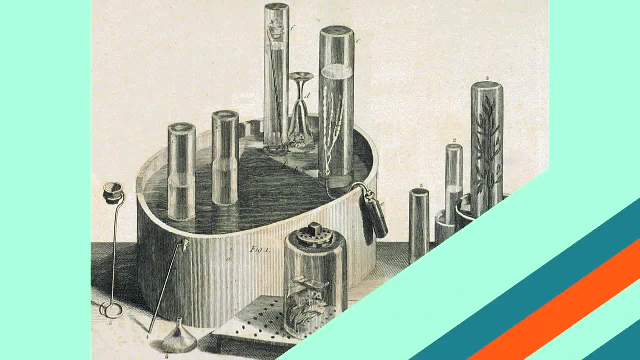 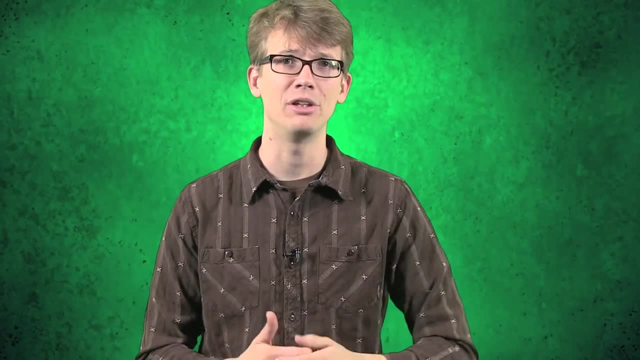 He basically just filled a bottle with water and inverted it in place, Then he turned it into a trough which was also full of water, And from that first bottle he ran a tube into another bottle in which he put various compounds he wanted to study. 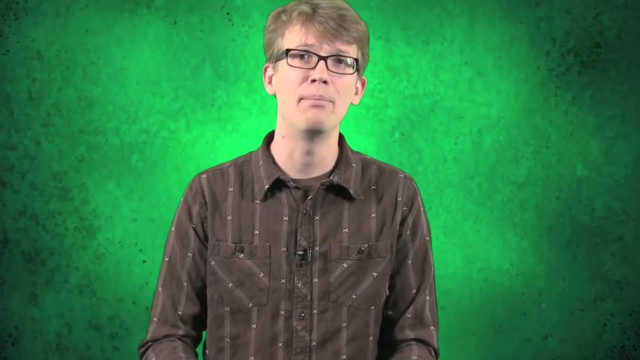 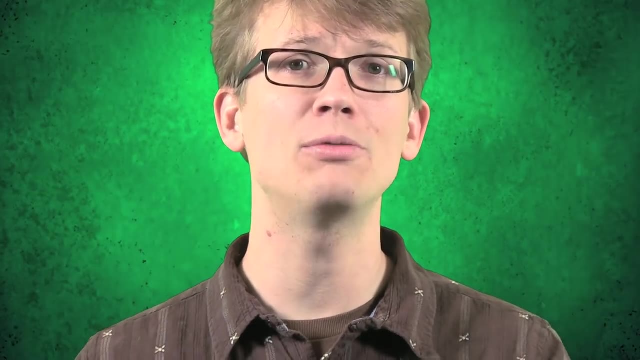 And then he heated them up. The gases released from the heating then bubbled up through the tube displacing the water inside the first bottle, filling it with gas. Priestley heated all kinds of stuff with this pneumatic trough, And in this way he discovered nitric oxide, hydrogen chloride. 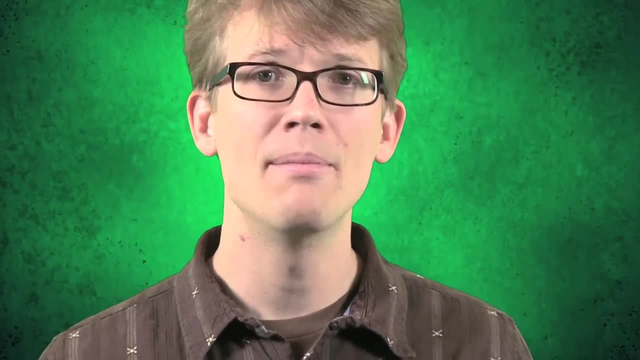 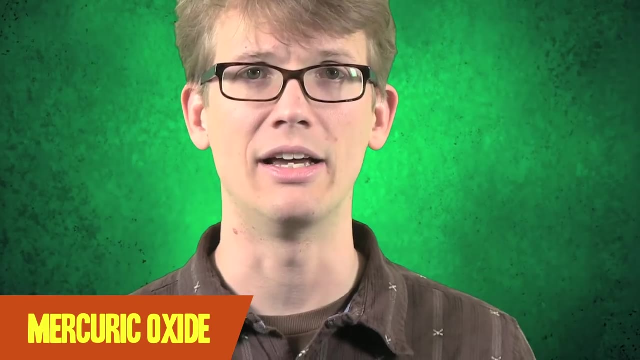 ammonia, sulfur dioxide and nitrous oxide, among others. But his most important discovery was oxygen, which he isolated by focusing a beam of sunlight on mercuric oxide. Being a true hands-on scientist, he took the bottle from his trough and huffed it. 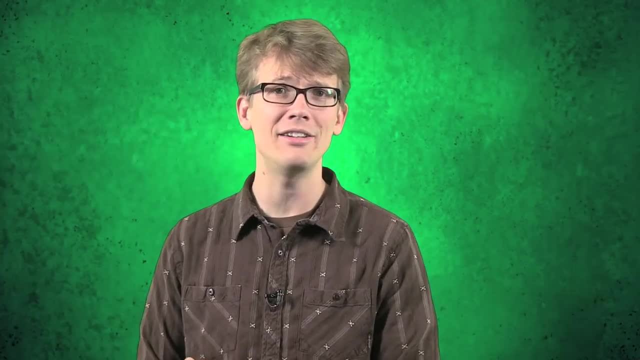 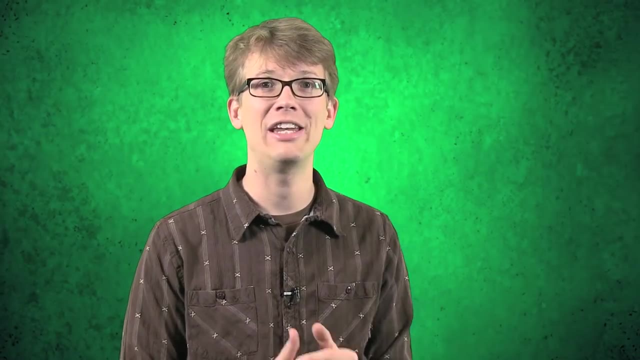 He said later, I fancied that my breast felt particularly light and easy for some time afterwards. Of course, he had no idea that he'd created the gas that we all need to like exist. He just thought that he'd removed the element of fire, or phlogiston, from the air. 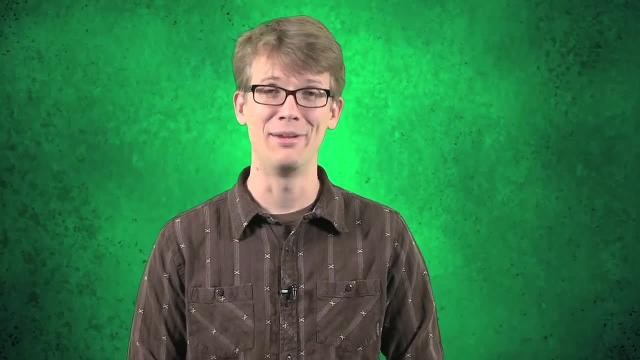 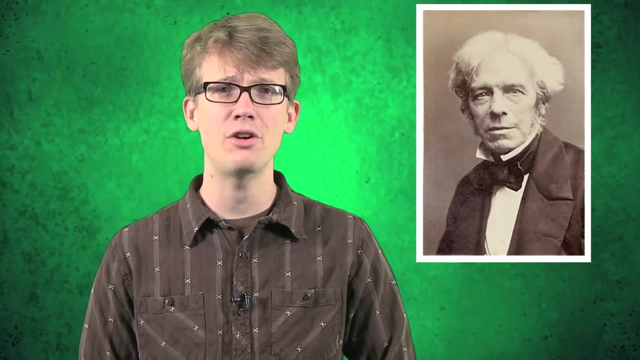 Yeah, he was still operating under the idea that fire was an element, But doing great chemistry nonetheless. Number two: the discovery of ions. Michael Faraday, a 19th century English scientist, has been called the greatest experimenter of all time. 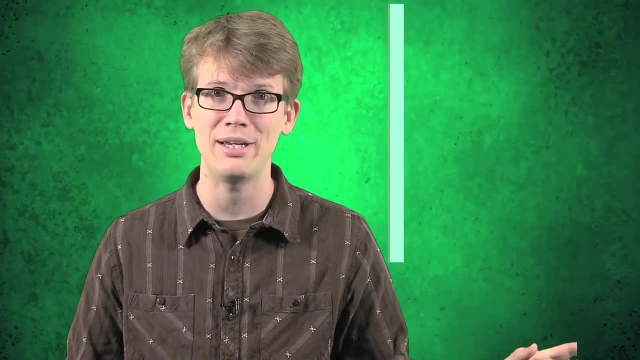 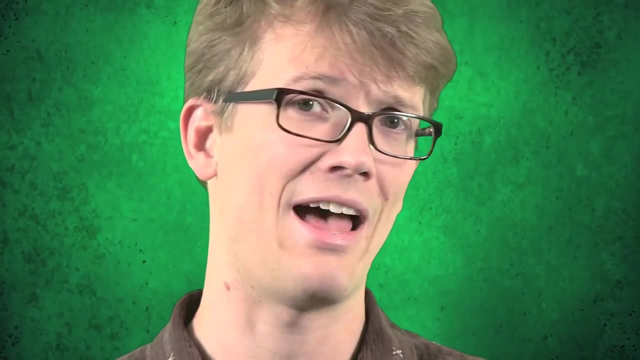 Albert Einstein had a picture of Faraday on his wall. Dude was big time, And though he wasn't just a chemist, he basically discovered electromagnetic fields and invented the first Bunsen burner and laid the groundwork for us to have electricity. he did discover ions, atoms with an electric charge. 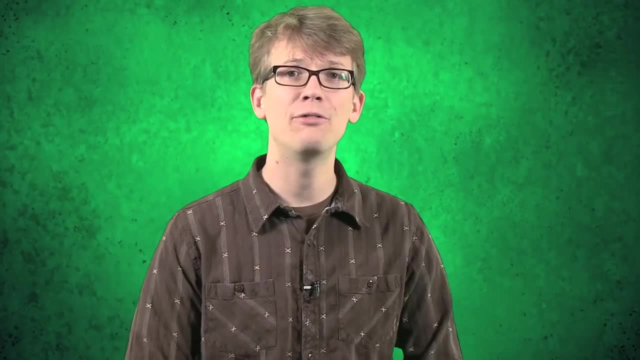 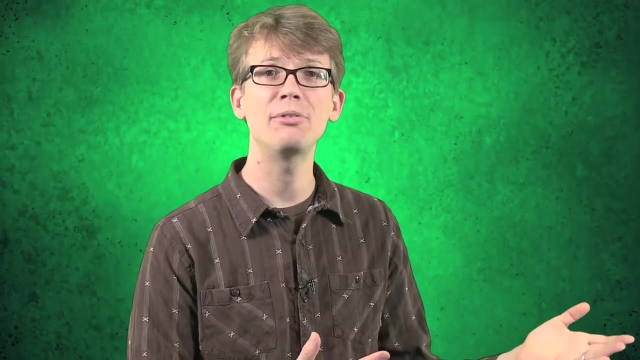 Faraday discovered ions as part of his obsession with electricity. In 1834, while he was messing around with electric current in water, he discovered that certain substances that were dissolved in water conducted a current. He didn't know precisely what was doing it, but he knew that some kinds of particles must 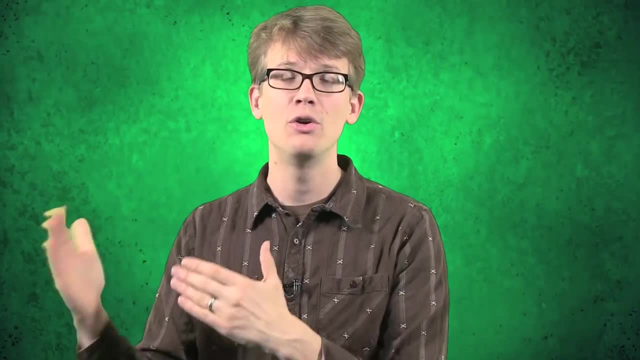 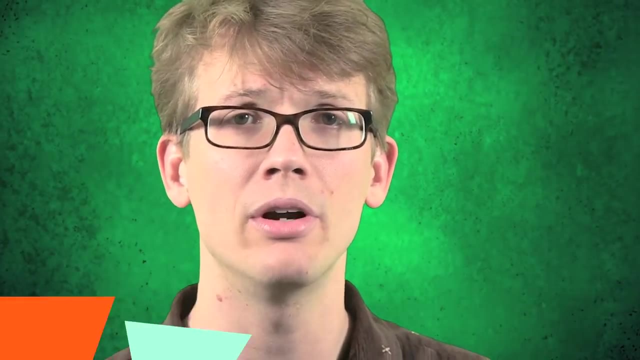 be relaying the charge through the water from one electrode to the other. Now, Faraday was great at discovering stuff, but he was terrible at naming the things that he discovered. so he wrote to a friend and mentor, William Hewell, who had coined quite 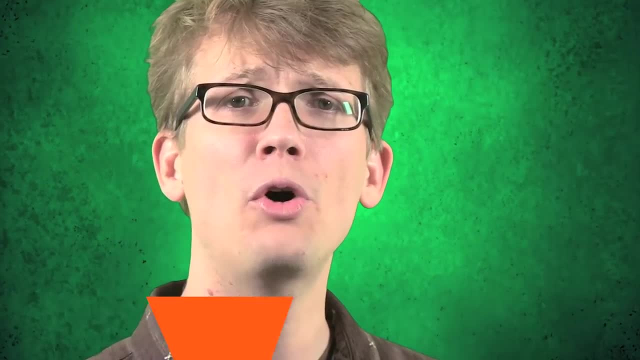 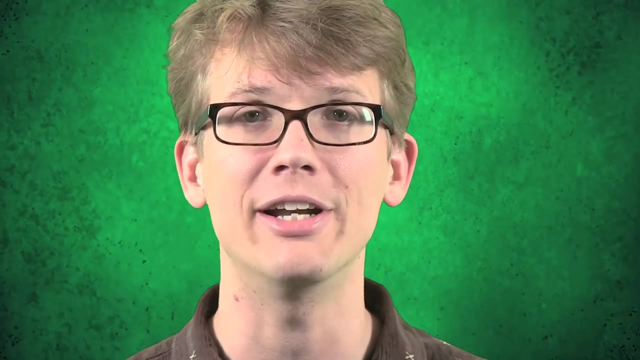 a few excellent terms in his time, including the word scientist. Hewell wrote back suggesting the name ions from the Greek word to go, which today we know are the things that swap electrons to create a current. Amazingly enough, all of this was done before electrons had even been discovered. 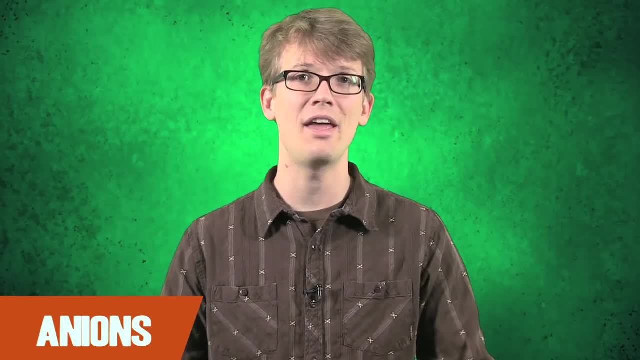 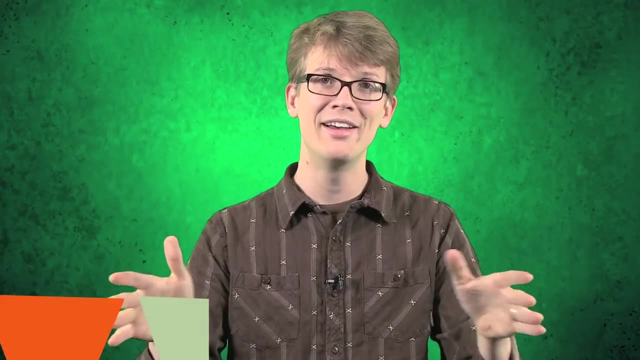 Faraday was even able to classify ions into anions or negative ions that were attracted to the anode and cations which were drawn to the positive electrode or the cathode. All of those words, by the way, coined by Hewell. 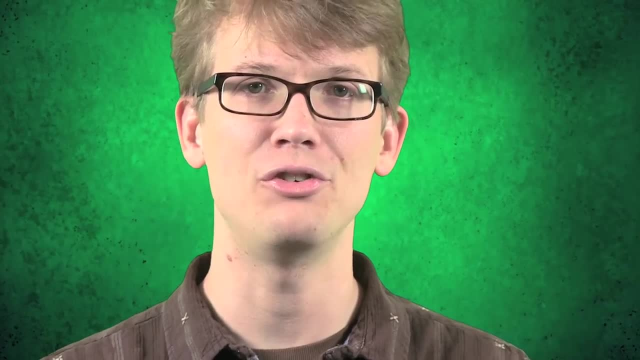 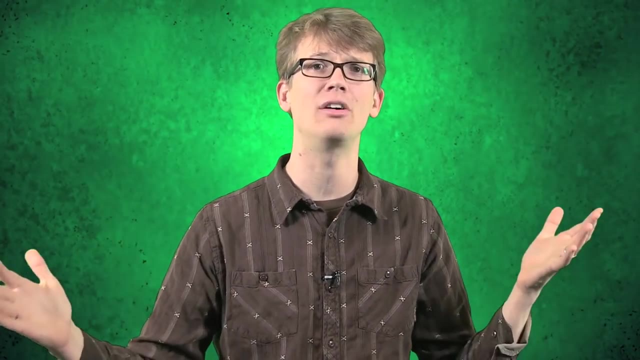 And finally, our number one experiment, the first synthesized drug. These days, scientists are constantly creating chemicals to cure what ails us. Our bodies are, after all, just a bunch of chemical reactions all happening at once, And when some chemical reaction makes us feel cruddy or brick or something like that, we can't do anything about it. And when some chemical reaction makes us feel cruddy or brick or something like that, we can't do anything about it. And when some chemical reaction makes us feel cruddy or brick or something like that, we can't do anything about it. 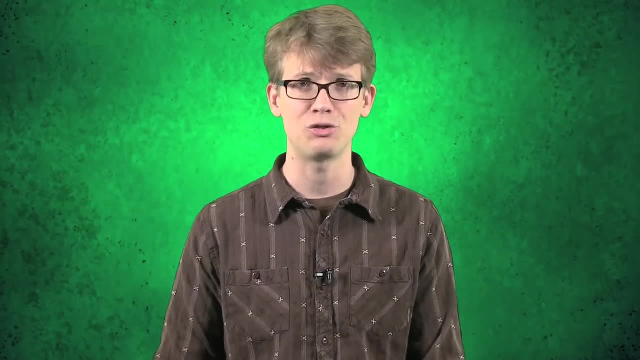 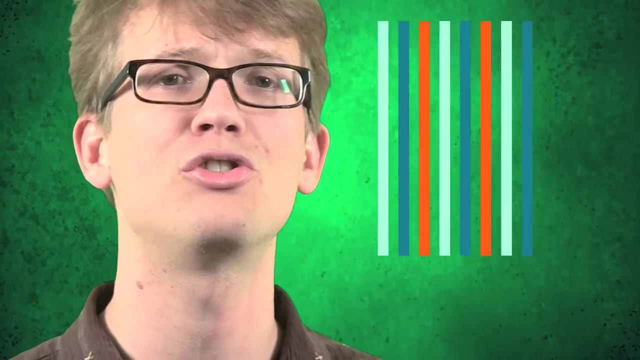 When something breaks down and doesn't function properly. we've figured out ways of setting things straight, And although humans have been doing this for hundreds of thousands of years with natural chemicals, it wasn't until 1853 that French chemist Charles Gerhardt synthesized acetylsalicylic acid, or aspirin. 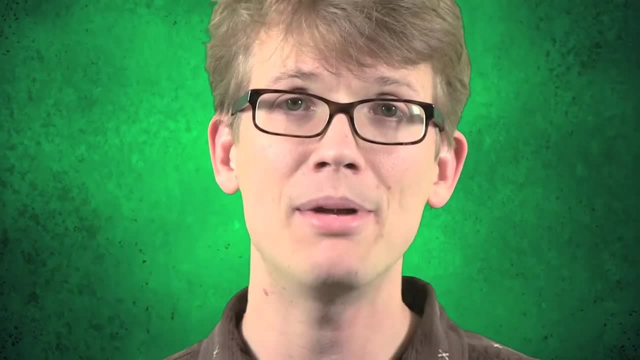 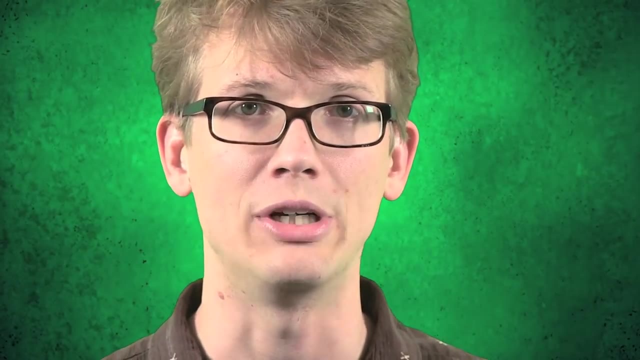 It wasn't until 1853 that French chemist Charles Gerhardt synthesized acetylsalicylic acid, or aspirin. He did it by mixing acetyl chloride with a salt of salicylic acid to create the same compound that you find in the bark of the white willow tree. 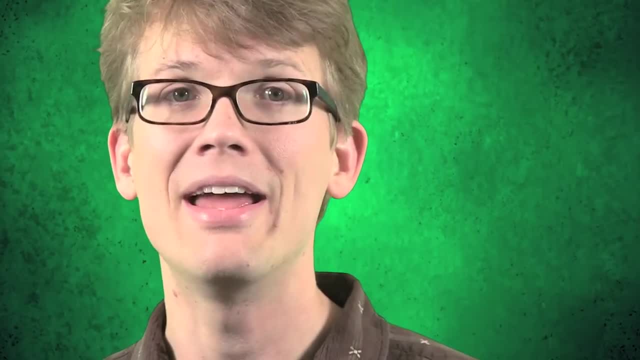 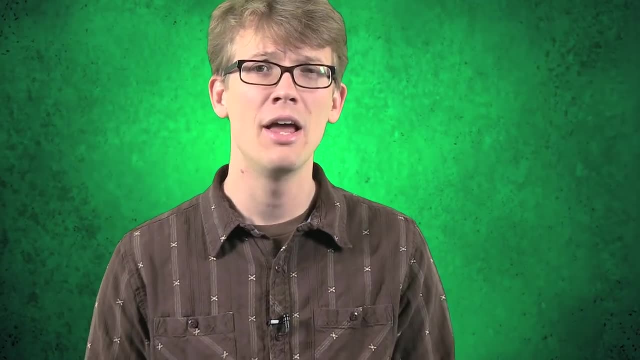 He was able to determine what compounds were in the willow bark and then create them in the lab. It's hard to underestimate the importance of this. Gerhardt's synthesis of this chemical based on high比 Alternating Testimony synthesis of aspirin in the Bayer Corporation's later improvement of that synthesis has probably altered the course of human history more than any other chemical reaction ever. Not because it helped our aches and pains- though that's a nice side effect- but because it showed that it's possible to use chemistry to cure people. This is something that no one fully understood at the time, but would lead to a huge increase. 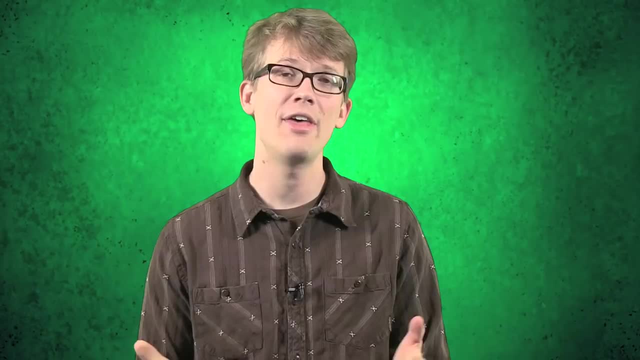 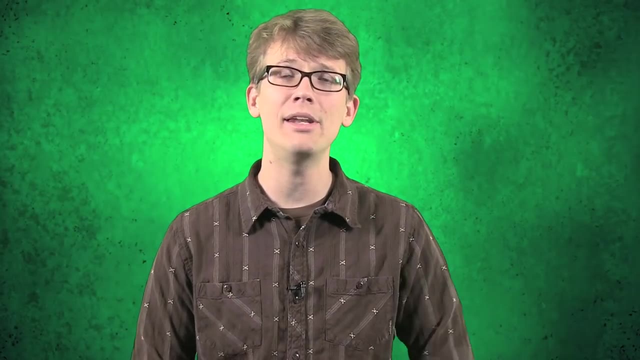 in the quality and length of human life. Not bad, Mr Gerhardt. Thank you for watching this SciShow Dose. If you have any questions or comments or ideas for us, we're on Facebook and Twitter and, of course, down in the comments below, and if you want to keep getting smarter, with us. 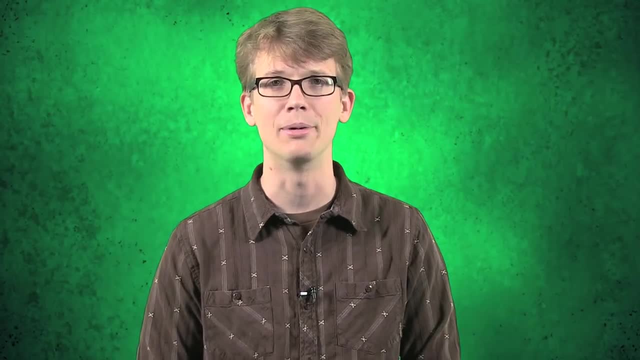 here at SciShow. you can go to youtubecom, slash SciShow and subscribe. 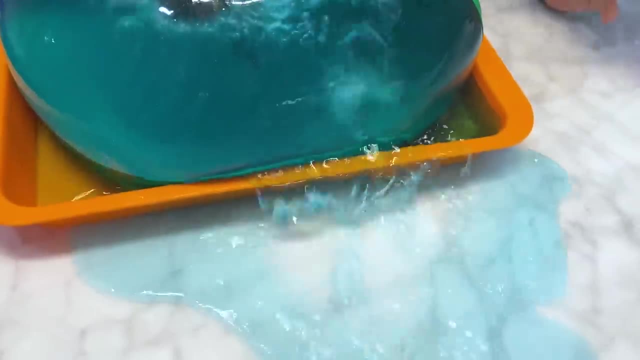 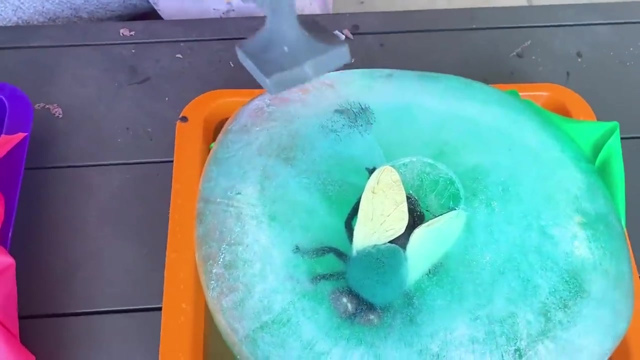 Wow, it's dripping already. Oh no, there's a leak. Okay, Emma's turn. It's not easy. huh, Emma, you broke it a little bit. You can do this. You can do this. Whoa nice. 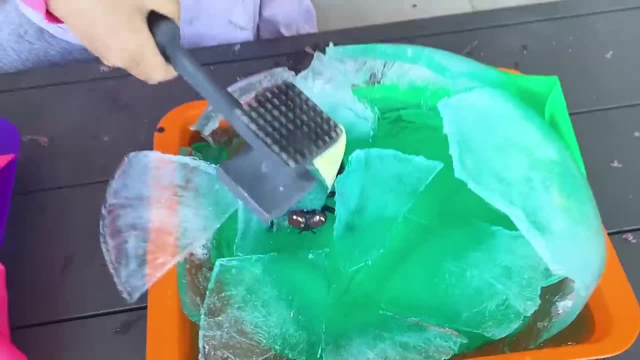 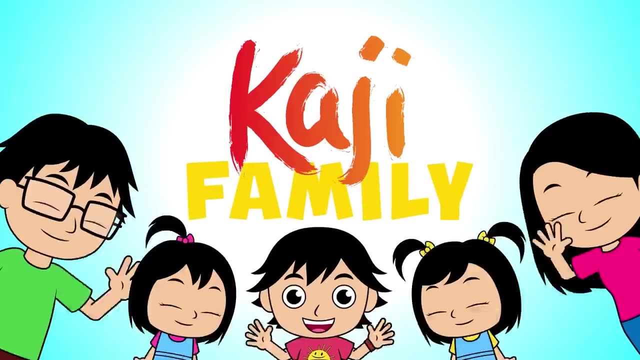 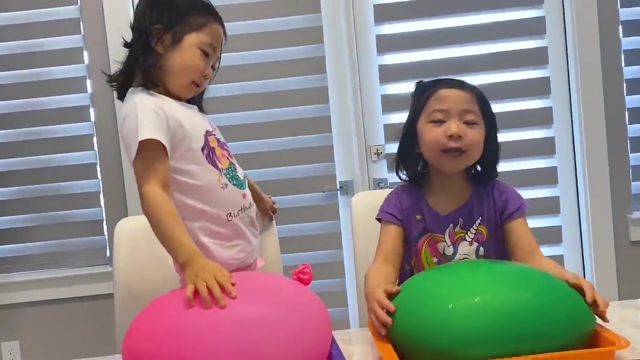 Whoa, Emma, you did it. You freed the fly. Yay, Good job, Emma. The fly is almost free. Hi Podgy Family, Hi Emma Kay. Hi Mommy, Do you know what we're doing today? Ice balloon.